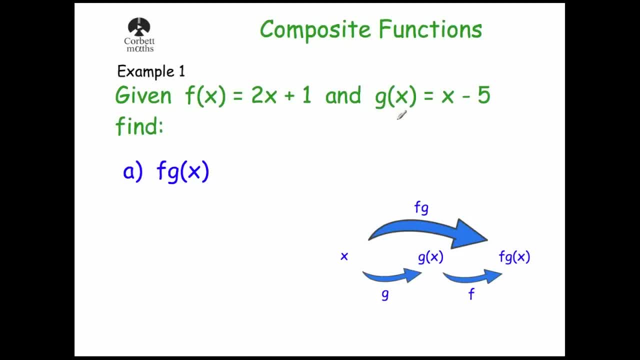 says: given f of x equals 2x plus 1 and g of x equals x minus 5, find fg of x. So here we've got x, We apply g first of all, and we get g of x, and then we apply f and we. 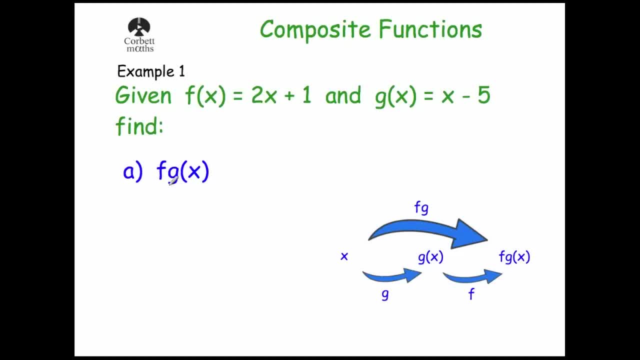 get fg of x. So what we want to do is: we want to apply, we've got fg, we want to apply g and then we want to apply f. So here we've got g of x and then we want to apply f. So 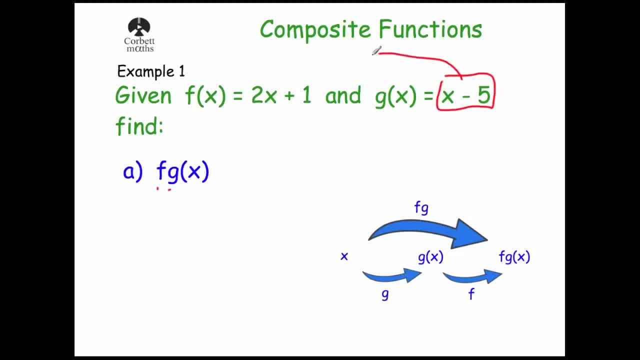 g of x. So if we take this x minus 5 and we put it into our f of x, in for the value of x here, we can then expand that and find out what our fg of x is. So what we're going. 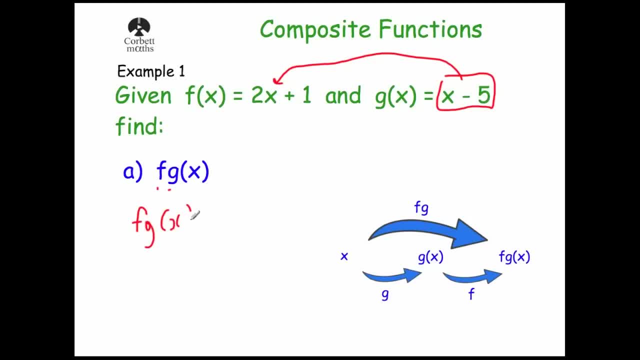 to do is we're going to write fg of x equals. now we look at our f of x function, which is 2x plus 1, but we're going to put in the g of x into that for the x. So we're going to. 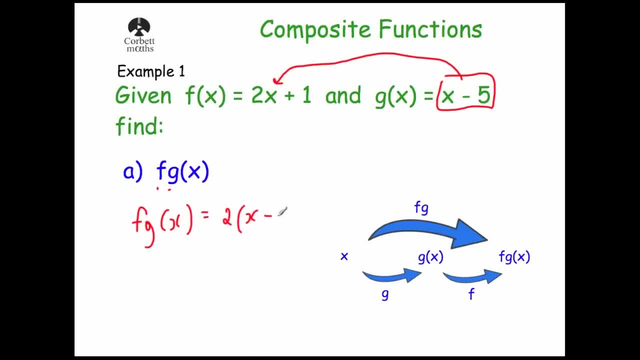 write 2 bracket and then we write our x minus 5 and then close brackets and then our plus 1.. And then whenever we expand that, well let's have a look at what we get. We get 2x minus 10 plus 1.. So overall that would be: our fg of x would be equal to 2x minus 9.. And that's. 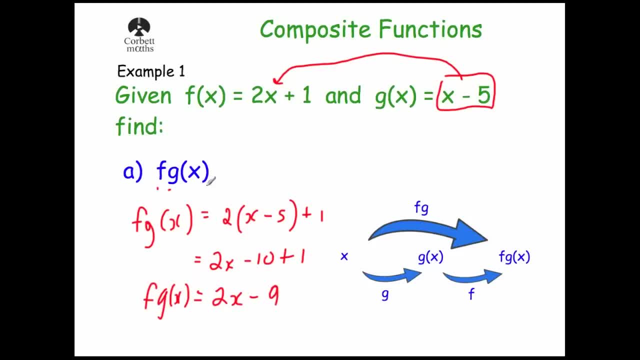 it. So that is our fg of x. Now let's just check it works. okay, Let's just choose a value for x. okay, So let's just say, for instance, x is equal to 2, okay, So we would apply g first of all to it. So 2 minus 5 would be equal to 2.. So that's it. So that's. 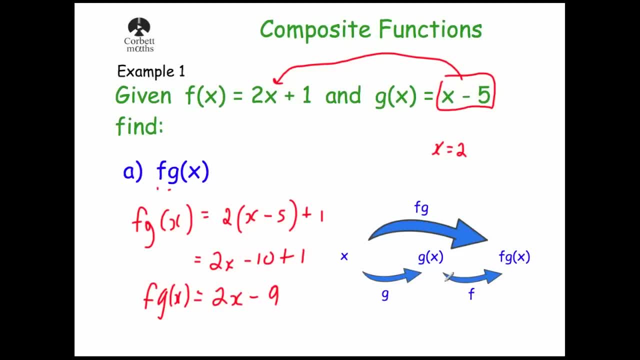 equal to minus 3.. And then we would apply f to it. okay, So we've got minus 3.. So 2 times minus 3 is minus 6 plus 1 would be equal to minus 5.. Now, if we just take our 2 first of, 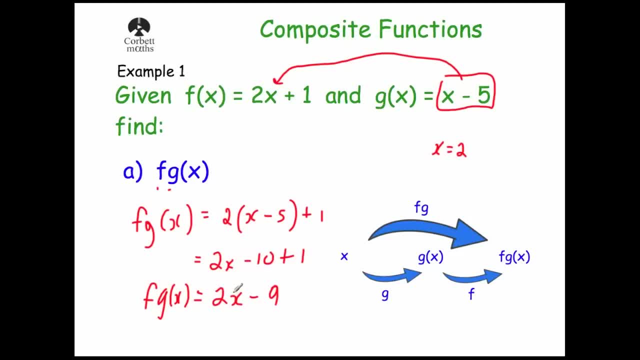 all and put it straight into our answer, we would get 2 times 2, which is 4 minus 9, which is also equal to minus 5.. So we see this function. rather than applying g and then f, we could just apply this function of 2x minus 9, and it will bring us to the same values at the end. okay, So if you want to find fg of x, we're going to use fg of x. So we're going to take fg of x and we're going to take fg of x, and we're going to take fg of x and we're going to take. 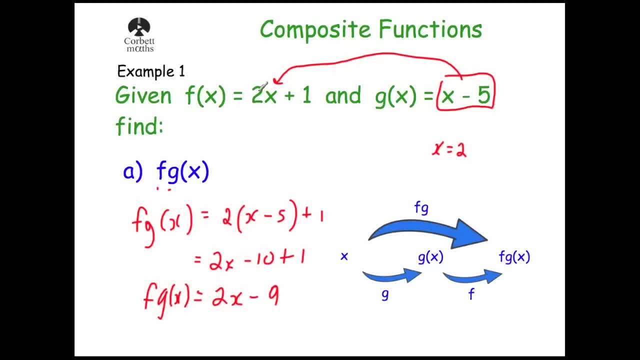 fg of x. You take your g of x and you put it into your f of x. Next Part b: This time we want to find g f of x. okay, So do you notice, the f is closest to the x. That means: 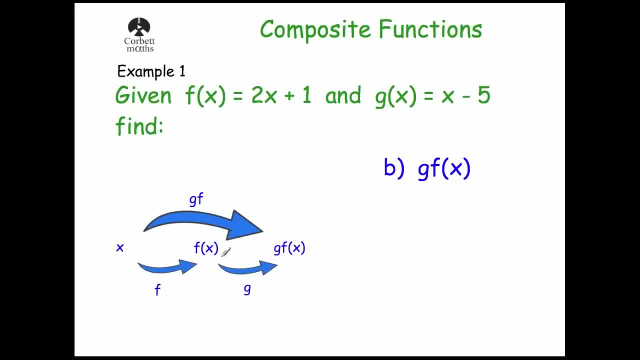 we're going to apply the function f first of all, and then we're going to apply the function g. okay, So this time what we're going to do is to find this overall, this composite function g, f of x. what we're going to do is we're going to take our f of x and we're 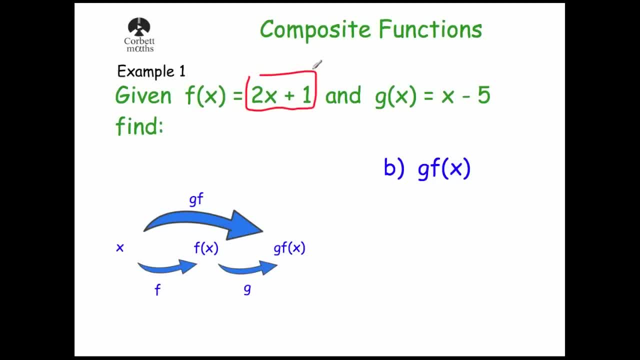 going to put it into g. So our f of x is this and we're going to put it into the function g there, okay, And put the value for x in the function, So g f of x will be equal to. well, it's x. 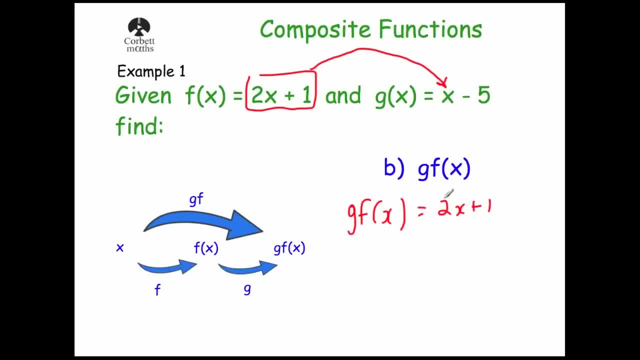 which is this, which is 2x plus 1, and then we're going to take away 5. Whenever we have that, well, we didn't actually need the brackets there, so we've got 2x and then 1, take away. 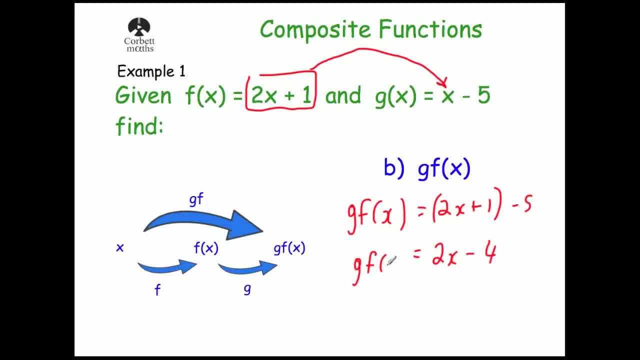 5, will be equal to minus 4.. So g f of x will be equal to 2x. Let's check it. So let's again say that x is equal to 2.. If we apply f of x, we're going to get f of x. 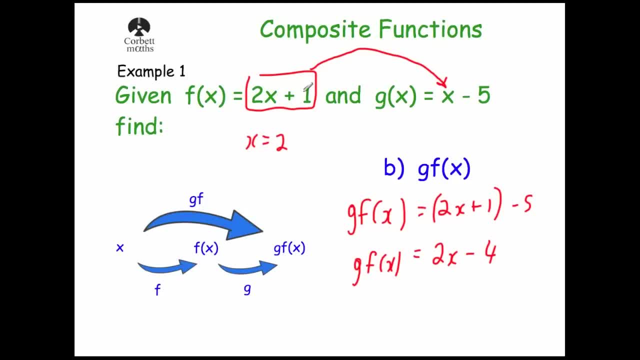 If we apply f first of all, well, f of x is 2x plus 1.. 2 times 2 is 4 plus 1 is 5.. And then we apply the function g, which is x minus 5, well, 5 minus 5 is 0.. So if we put in 2,, 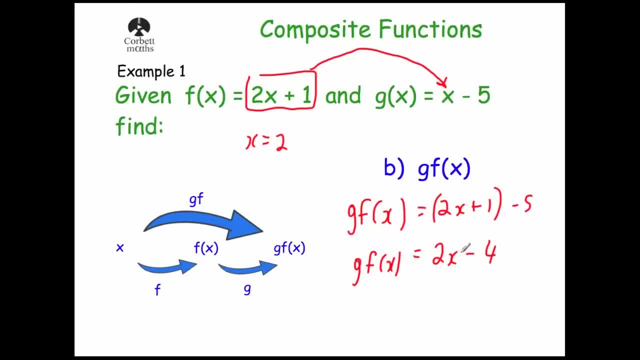 we get 0.. Let's try it with our composite function: 2 times 2 is 4, take away: 4 is 0. So it shows you that it works okay. So if you want to find g f of x, you take your f. 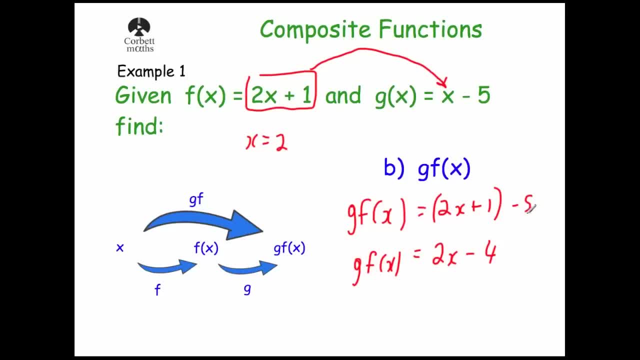 of x and you put it into your g of x. Okay, let's try some examples now, and we'll do it without the use of this diagram. So example two: given f of x equals x squared plus 2 and g of x equals 2x plus 1, find f. 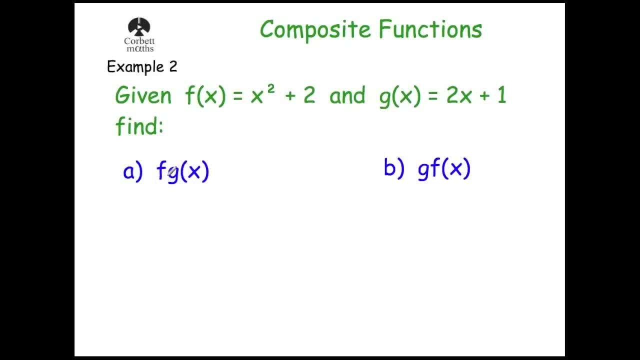 g of x. So if we want to find f g of x, we're going to take our g of x and put it into f of x. So we want to take our g of x and put it into our f of x here. okay, in for the value for. 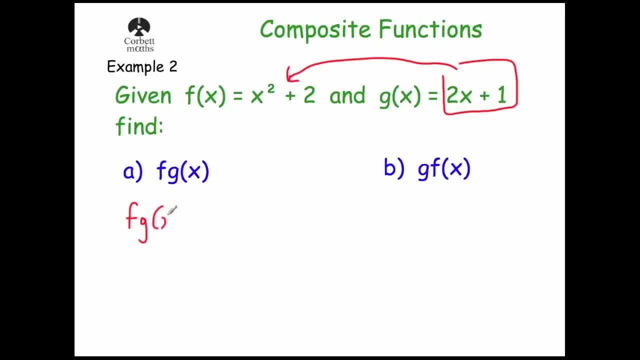 x. Okay, so f g of x will equal. well, our f of x is x squared, but instead of x squared we're going to put our 2x plus 1.. Close that out. So we put in: our g of x equals 2x plus 1.. So f g of x equals 2x plus 1.. Find our f g of. 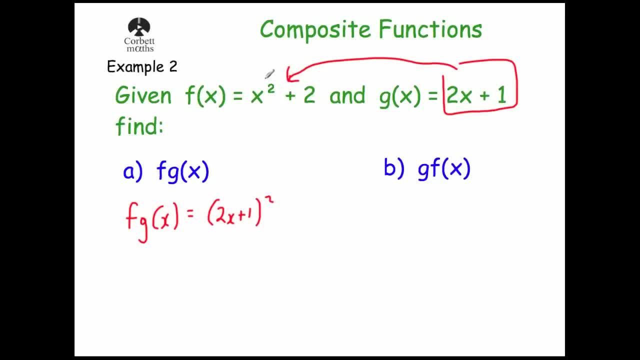 x bracket squared and then we have our plus two. so we then write plus two. so in other words, we just replace the value for X or the X with our G of X function. so now we're going to need to expand this. so if we expand it, remember we've 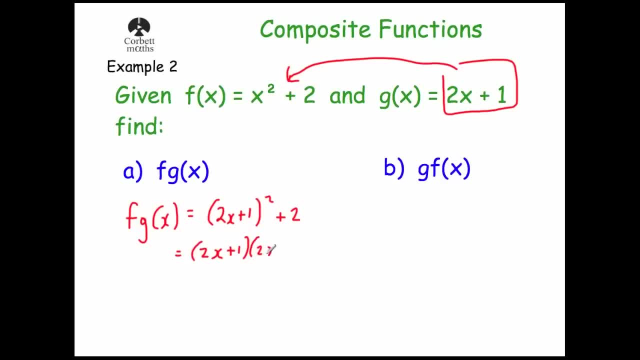 read the bracket out twice, so 2x plus 1, 2x plus 1, and then write our plus 2 on the end using FOIL: expanding this would give us 4x squared plus 2x plus 2x plus 1. and then don't forget our plus 2 on the end. so we would get FG of X would be. 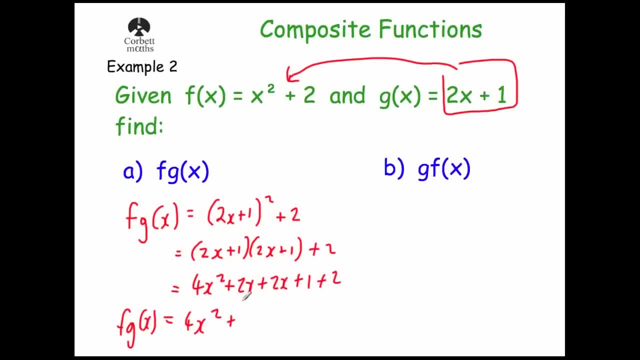 equal to 4x squared plus 4x plus 3, and that's it. that's our composite function FG of X. this time we're now going to find G, F of X. so we're going to take our F of X and we're going to put it into the function G. 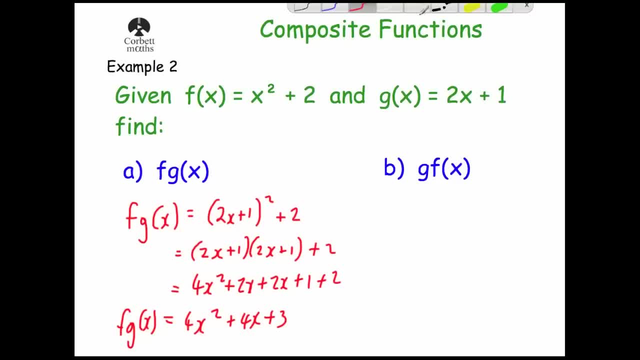 so let's just put that out. so we're going to take our F of X now we're going to put it replace the, the X in the function G with that. we're gonna put it in there. so G, F of X would equal, or two, and then our bracket, our x squared plus. 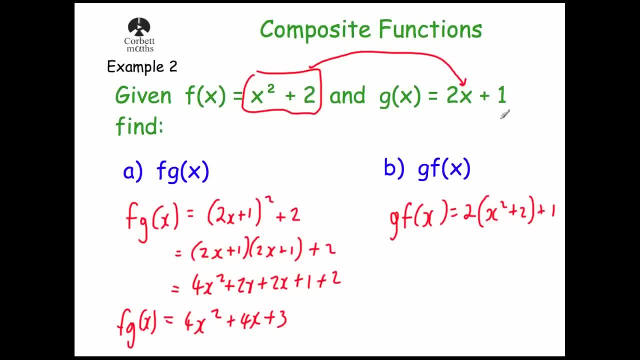 2 instead of the X and then plus one on the end. so whenever we expand that, we get 2x squared plus four, and then our our plus 1, so which should give us 2x squared plus 5, and that is our g f of x, and that's it. 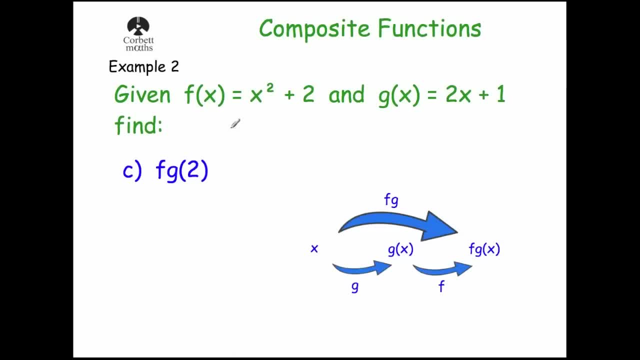 okay, so let's have a look at part c. like functions such as f of x and g of x, with composite functions you can substitute values in for the variable, such as fg of 2. so what that means is we're going to put 2 into fg, that composite function. okay, so we've worked out fg. 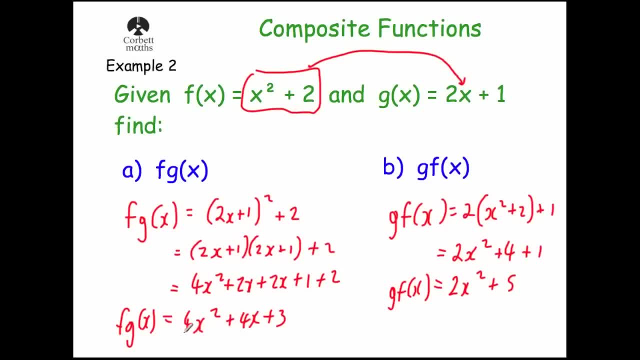 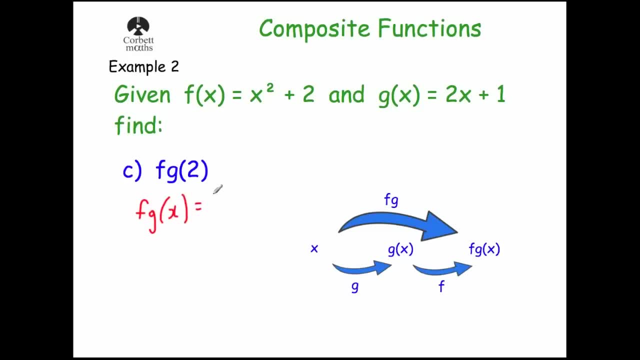 previously, just a second ago, and fg of x was equal to 4x squared plus 4x plus 3. so fg of x is equal to 4x squared plus 4x plus 3. so that's the composite function. now, as you can see, we're. 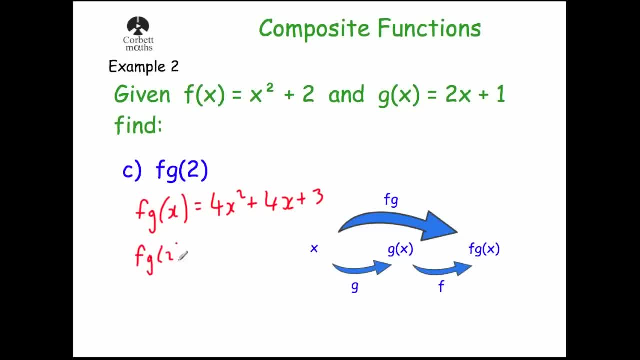 going to substitute in the value 2 here. so fg of 2 would equal 4 times 2, squared, remember, with bob mass. we're going to square that 2 first of all, plus 4 times 2 plus 3, so that will give us 4 times 4 plus- let's work this bit out- 8 plus 3, 4 times 4, 16 plus 8 plus 3. 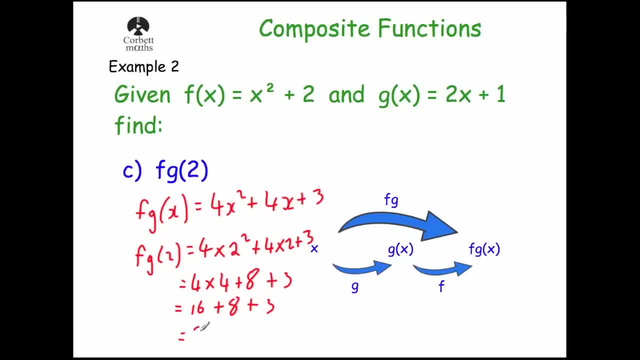 16 plus 8 is equal to 24 plus 3 would be 27, so fg of 2 is equal to 27. now, if we didn't know that composite function, you can do it using the two individual functions g of x and f of x. and 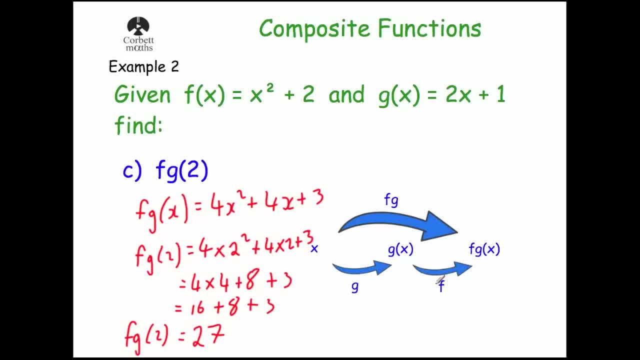 just remember that fg means you apply g first of all and then you apply f. so we take our 2 and put it into the function g of x, so it would give us 2 times 2, which is 4, plus 1, which is 5, and then we put that into our f of x, which so it'd be 5 squared, which is 25 plus 2. 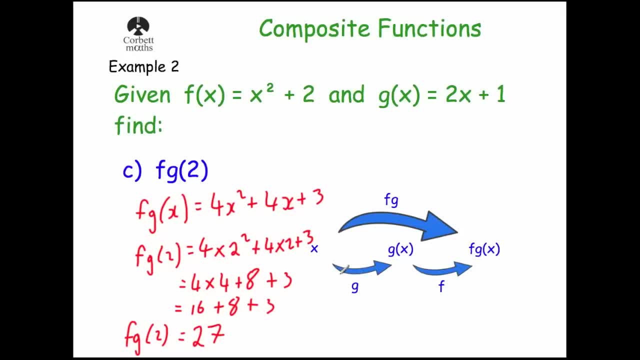 you'd also get 27, so you can do the two individual uh functions, uh, g of x and f of x, or we could just use the composite function um f, g of x. okay, part d, part d is to work out g, um g, f of 3. so 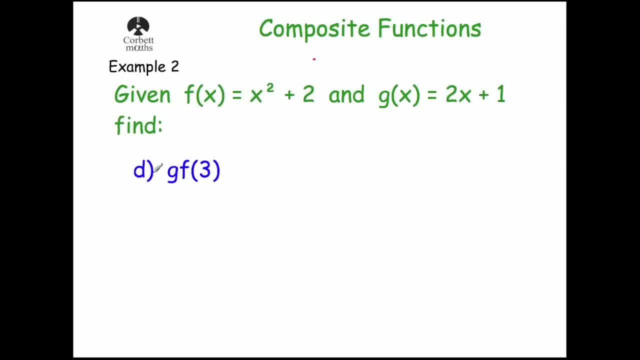 again. we could put the 3 into f of x and then get that answer and put it into g of x, um, or we've got the composite function here anyway, which is 2x squared plus 5, so g f of x is equal to 2x squared. 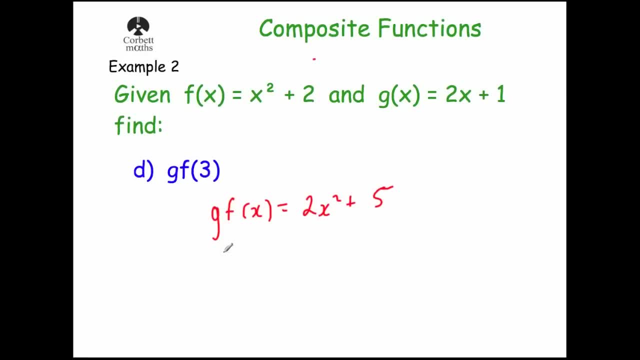 plus 5 and we're going to substitute in the value 3. so g f of 3 will equal 2 times 3 squared plus 5. well, 2 times 3 squared is 9 plus 5. 2 times 9 is 18 plus 5 would give us: 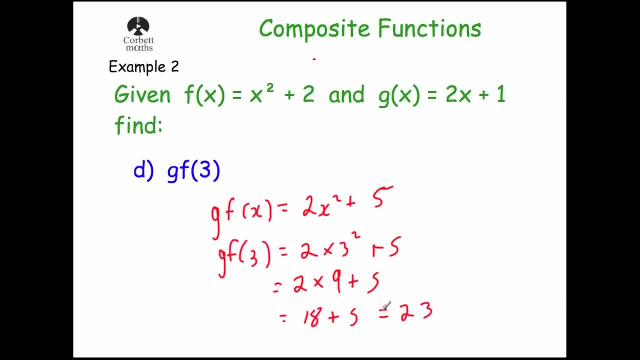 25. so that means that g f of 3 would be equal to 23. um, just to sort of show you, you can put it the 3 into f of x first of all. so 3 squared is 9 plus 2 is 11, and then get that and put it into g of x. 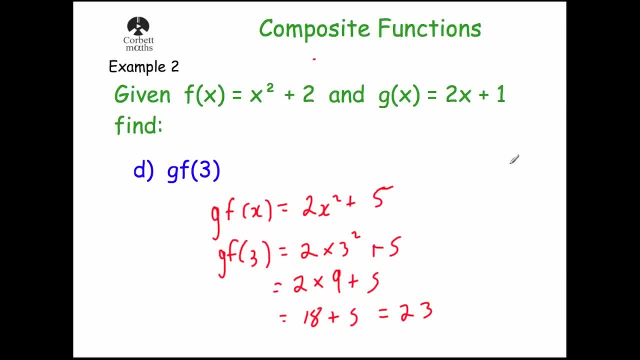 2 times 11 is 22 plus 1 is 23. okay, um. and example 3. example 3 says f of x equals 2x minus 1 and g of x equals um x plus 3. find the value of x, such as. 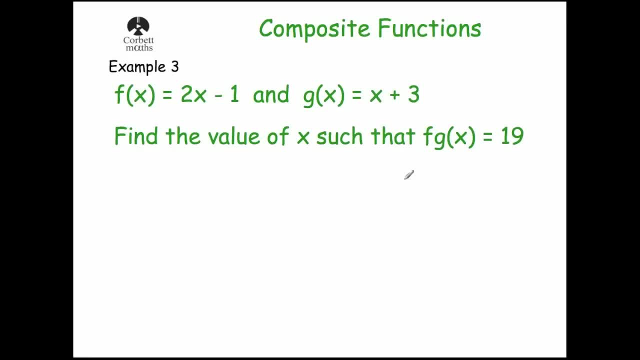 f of x equals 2x minus 1 and g of x equals um x plus 3. find the value of x, such as f of x equals g of x is equal to 19.. so we need to work out our fg of x. so we're going to put our g of x. 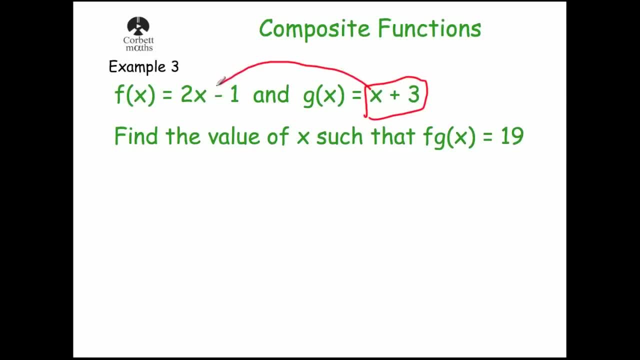 into our f of x, in for the value of x or in for x. so that would mean that fg of x will equal 2 bracket x plus 3 close brackets minus 1. that will give us 2x plus 6 minus 1, and that then 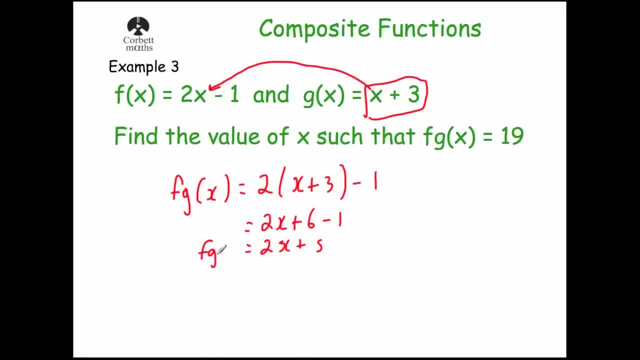 would be 2x plus 5, so fg of x is equal to 2x plus 3 minus 1, and that would give us 2x plus 6 minus 1, and that then would be 2x plus 5. so fg of x is: 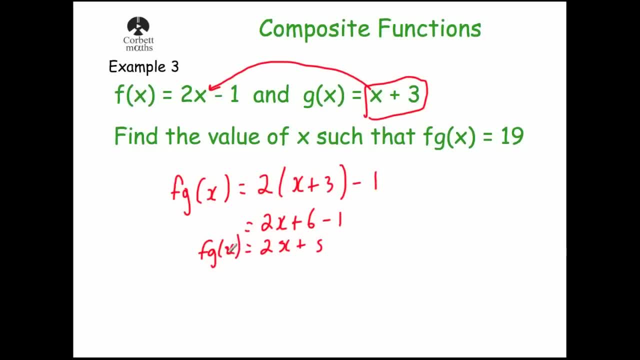 equal to 2x plus 5. now we know that that's equal to 19 and we want to find the value for x. so we're just going to make an equation, we're going to get our 2x plus 5 and just write: that's equal to 19. 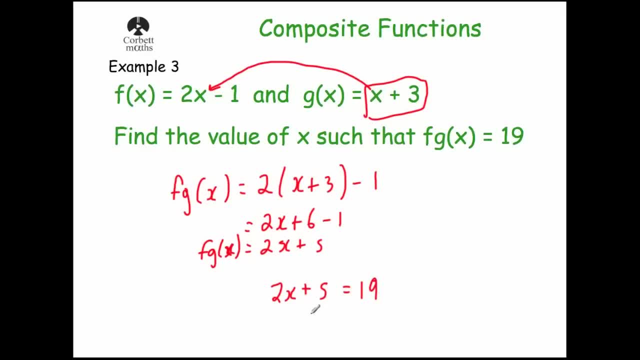 because we know it's going to be equal to 19, and find what x is. so minus 5 from both sides will give us 2x equals 14. divided by 2 mean that x equals 7, and let's just check it. if we get our 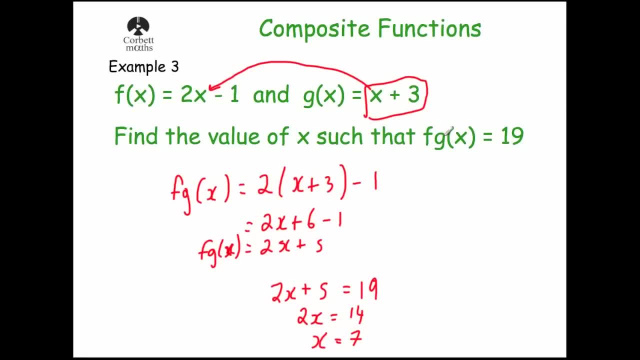 7. well, let's actually do it using the individual functions g of x and then f of x. put the 7 into the g of x, which would be 10, and then put that into f of x. 2 times 10 would be 20. take away 1. 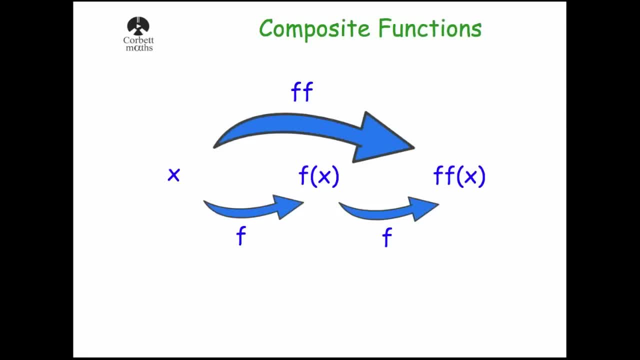 is 19, so that's it okay. and just to show you that sometimes you might see a function called f- f of x- or g- g of x- and what that means is you're just going to put f of x into f of x, so it means you're. 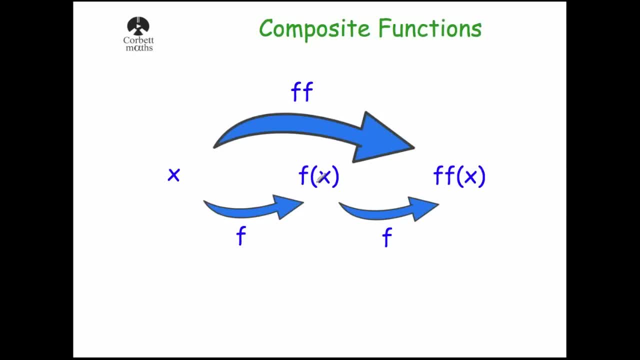 applying the function of, you're applying the function f and then you're going to apply it again, okay, so let's have a look at a quick example like that. so, given f of x equals 3x plus 5, find f, f of x. sometimes you might see it written as f squared of x and that means f, f of x. and then we need to. 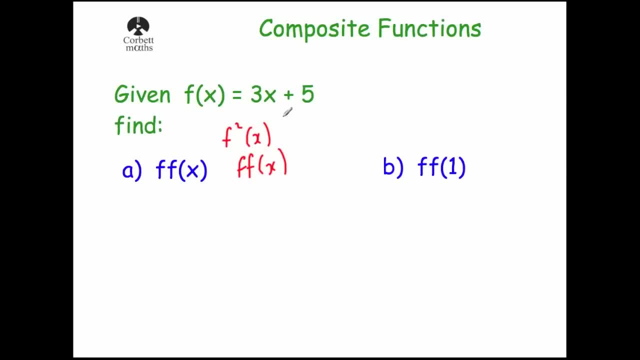 find f, f 1. so we're going to put our f of f, f of x into f of x. i'm just going to write it again so we can see it. so we're going to put our f of x here in for the value of x in the f of x there. 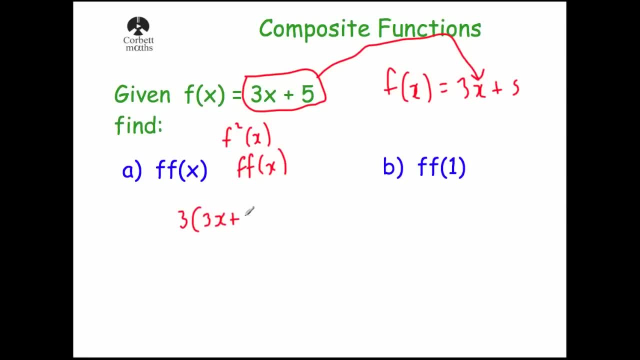 so 3 bracket, 3x plus 5, close brackets plus 5, and that would be f? f of x. well, that's it. that would be 9x plus 15 and then plus 5, so it would be equal to 9x plus 20, and then our f? f of. 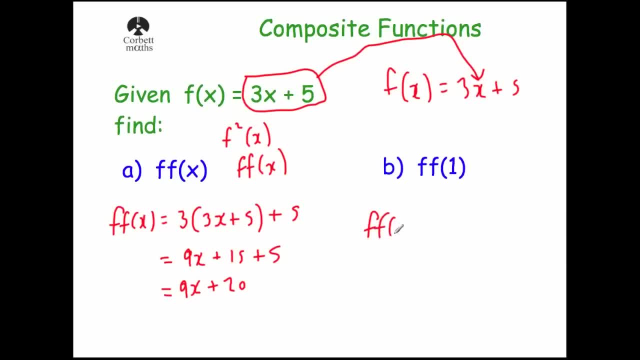 1. well, we just need to put 1 into that. so, given that f? f of x is equal to 9x plus 20, we're going to put 1 into that. so f? f of 1 would be equal to 9 times 1 plus 20, so it's going to be equal to 9. plus 20, 29, that's it. 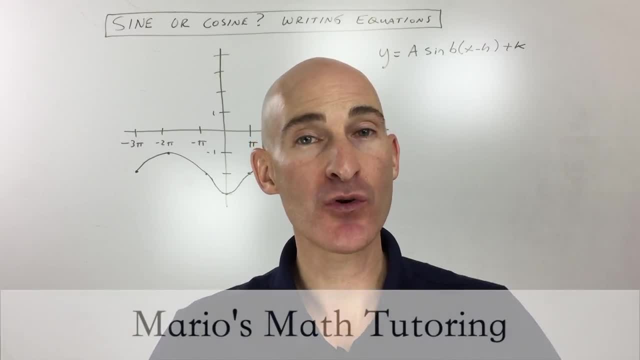 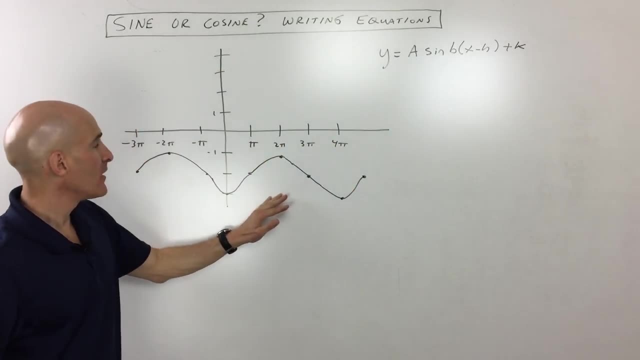 In this video you're going to learn about whether to use a sine equation or a cosine equation when you're describing a sinusoidal graph. So let's talk about some examples here. This first example: you can see: they give us a sinusoidal graph. What's a sinusoidal graph? Well, it's basically. 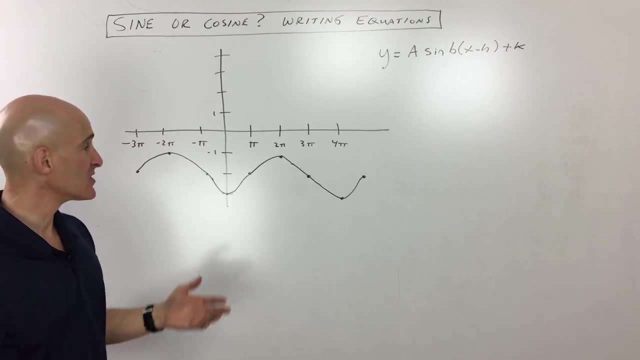 you know this s-shaped graph And this question that students always ask is: you know, do I use a sine equation or a cosine equation? And I'm here to tell you that you can use either one. Now the next question will say: well, do I use a positive, a value, or a negative, a value? And 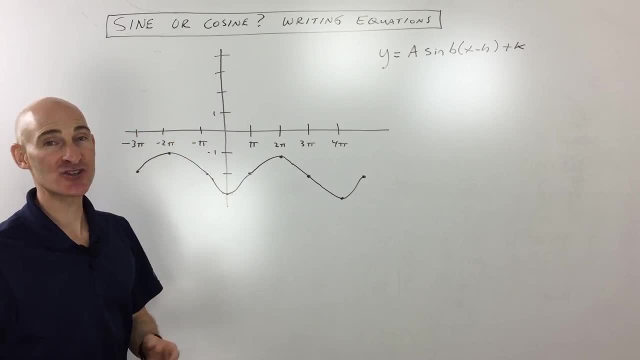 again the question is: the answer is: you can use either one, And I'll show you how to write these equations several different ways. The first thing that I would do is I would sketch in this midline. Now, when I say midline, what that means is: you know, it's the line that essentially 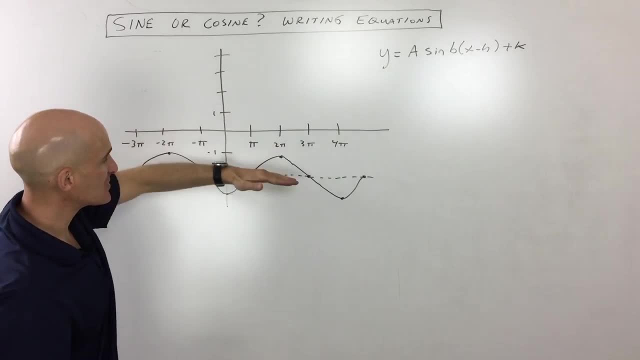 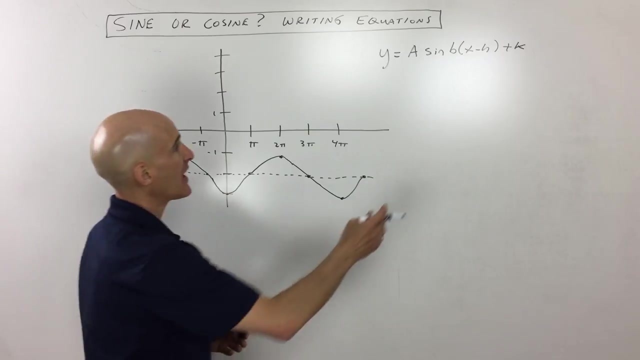 splits this graph in half, You've got half is above and half is below. That'll help you a lot. So what that tells us is what the vertical shift is. In this case, the graph is shifting down two. So no matter what equation that we write, it's always going to have a k value or a vertical.